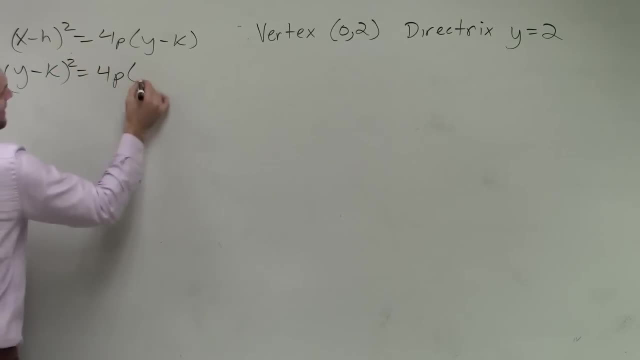 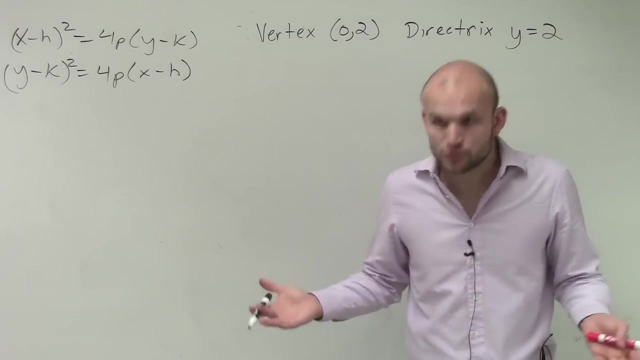 y minus k squared equals 4p x minus h. So there's two different equations we could hold on to. There's two different equations, guys, we could use. So how do we know which one to use right And which ones can help us find the standard form? So the best thing I like to do is to say: just plot what information they're giving you right. Because remember, when we were doing, we were finding the directrix and the focus. the first thing I asked you is: what's squared, the x or the y? When you know the x is squared, it opens up or down. When the y is squared, it opens left or right. 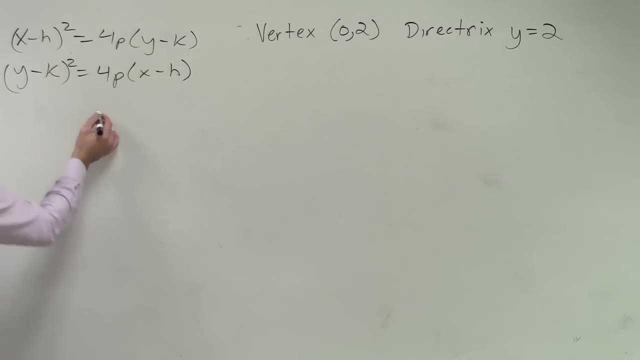 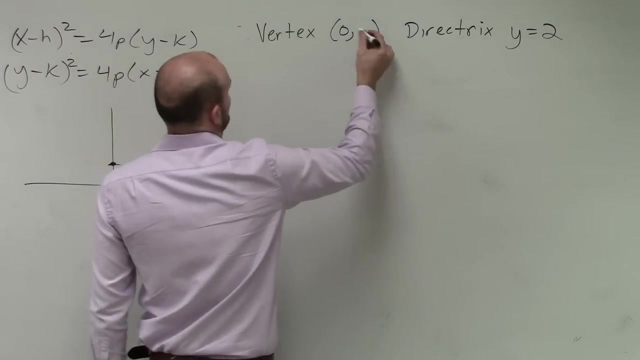 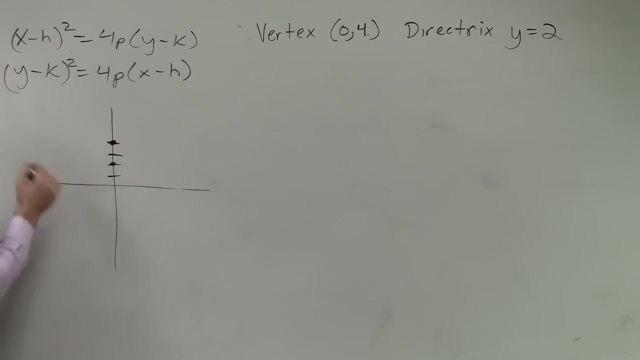 Correct. So let's go ahead and just graph what we have. So we have a vertex at 0, 2.. Then we have a directrix at whatever Vertex is at 0, 4.. So my vertex is at 0, 4.. Directrix is at 0, 2.. Okay, Well, obviously the laser is going to win First of all. 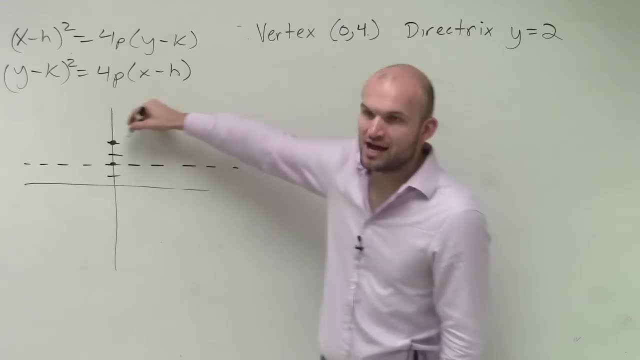 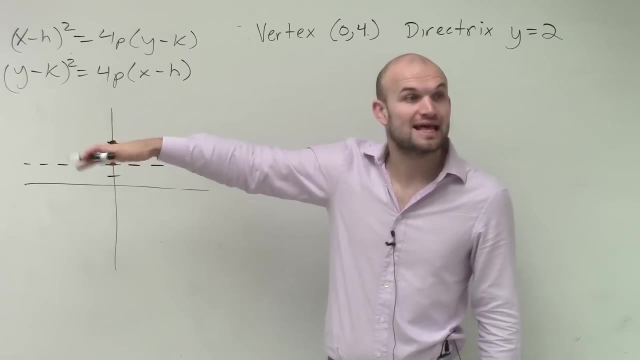 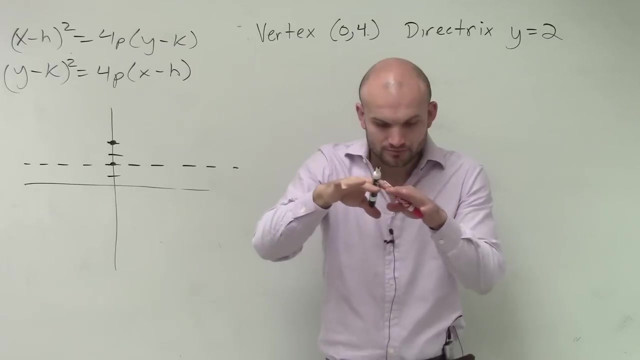 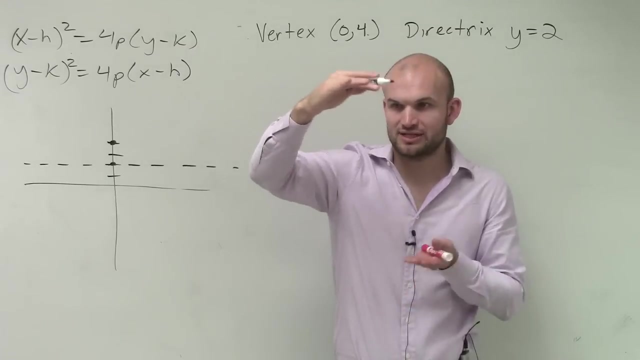 since we now know we have a horizontal, does our graph cross the directrix? Yes, It goes the opposite right. No, it's not going to go down because your, your, your, remember, your focus is inside your parabola and your directrix is opposite to being outside the parabola, right, Because they're the exact same distance. So we know our graph can't open down. And if it opened, to the right or to the left? 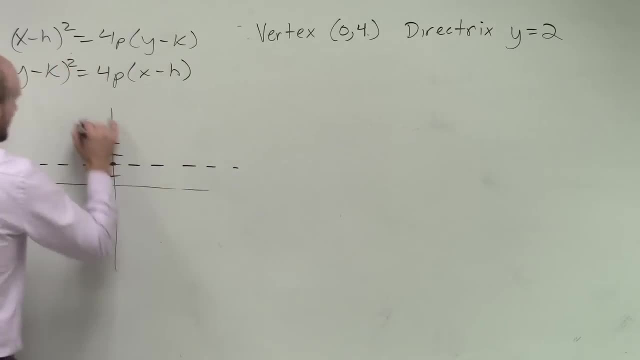 then it crossed the directrix as well. So the only possible point for us to do is have and to say that, oh, my graph has to open up, right, It's always going to go in the opposite direction of your directrix, And if your directrix is horizontal, then you know your graph has to open up. It can't open left or right, Right, Yes, Yeah, Okay. So now, how do we find the value of p? Well, ladies and gentlemen, remember: 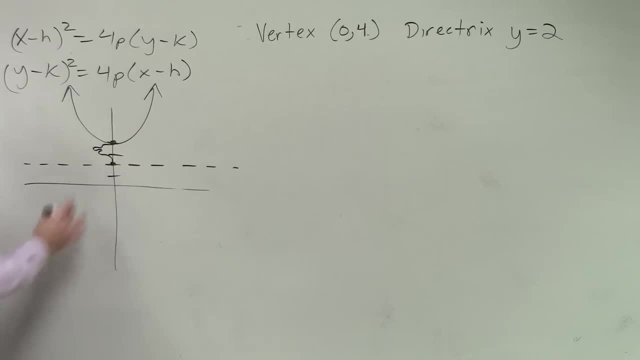 that this distance- I don't know what that is- This distance is the same, right here. So this distance, we count what? One, two units? Then we know that this distance has to be two units as well, Right, But since to find my, so remember, this is to your directrix And this is to my focus, which, here is my focus. 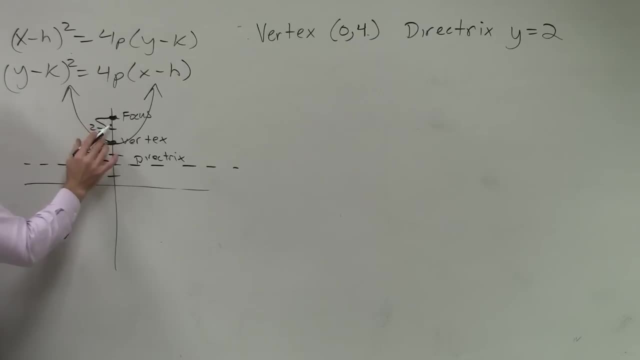 And this is to my vertex. So if I'm going up two units to get to my focus, right, And really I'd have to go down two units to get to my directrix. When I go up two units to get to my focus, I know now the p value is equal to what. 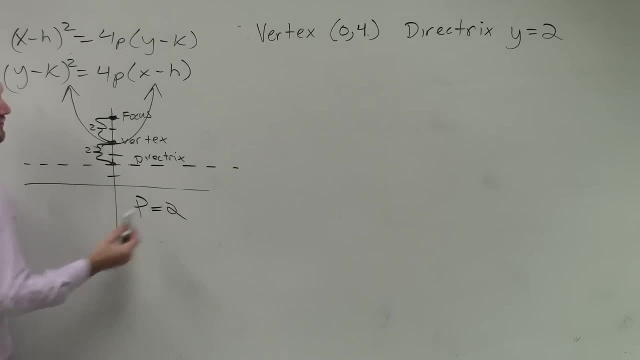 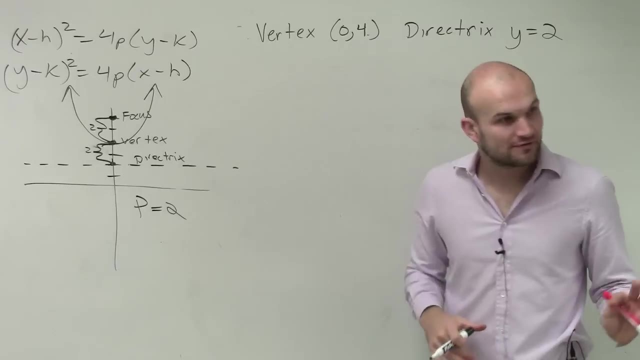 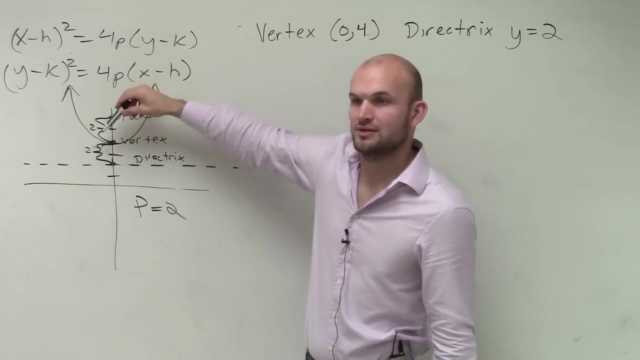 Zero, Zero. Remember, ladies and gentlemen, the value of p. the value of p- if you want to write this down, write it down. The value of p is the distance from your vertex to your focus. It can be anything. 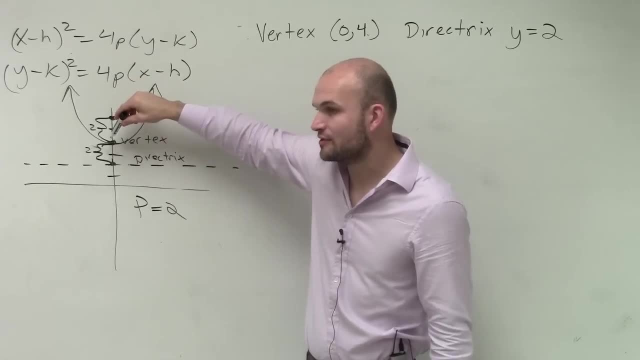 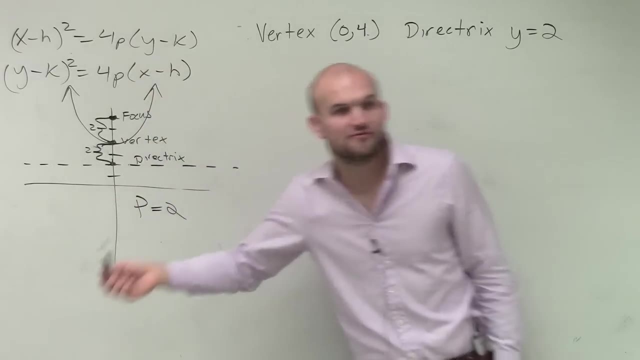 It can be positive, It can be negative, But it's the distance from your vertex to your focus. It doesn't matter if it's vertical or if it's horizontal, It's that distance from your focus to your vertex, or say, your vertex to your focus. 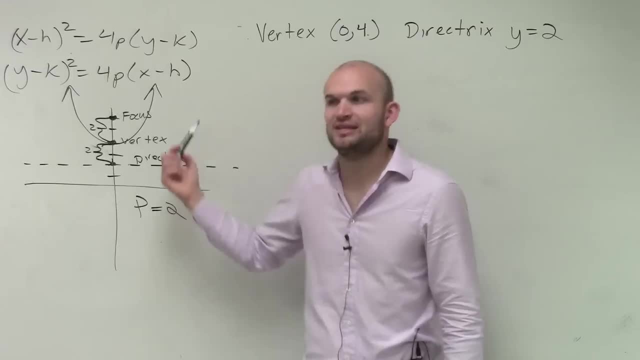 And then remember to go from your vertex to your directrix is going to be that exact same distance in the opposite direction. Okay, All right. So now we know that the graph opens up or down, So which formula am I going to use? 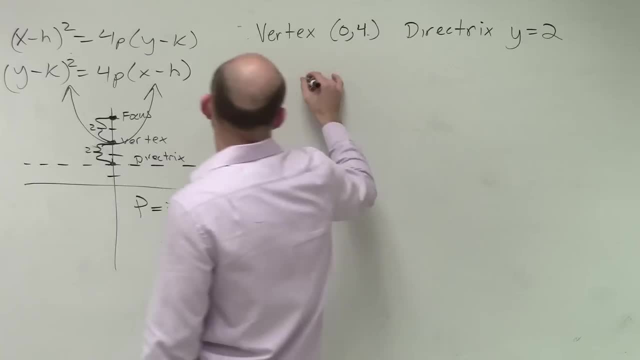 x squared or y squared, x squared, x squared right. So you do, x minus h squared equals 4p, y minus k. So now let's just plug in what we know. We know the vertex is 0, 4.. 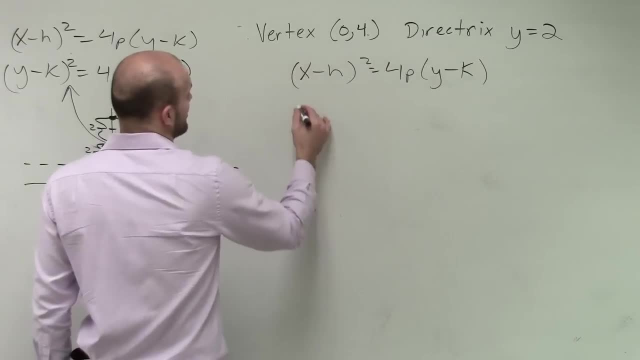 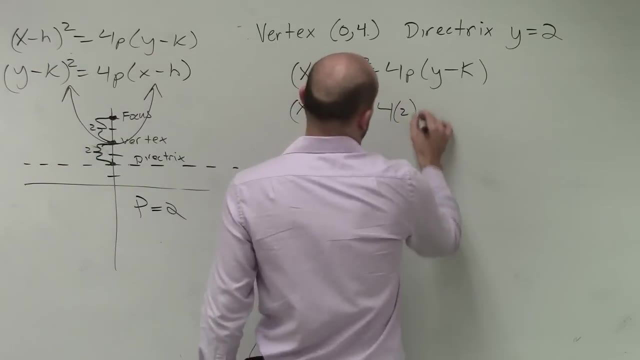 Remember it's opposite 0, 4.. So we have x minus 0 squared equals 4 times p, which we said was 2, times y, opposite of 4.. But there, So now we need to just write this in our standard form.